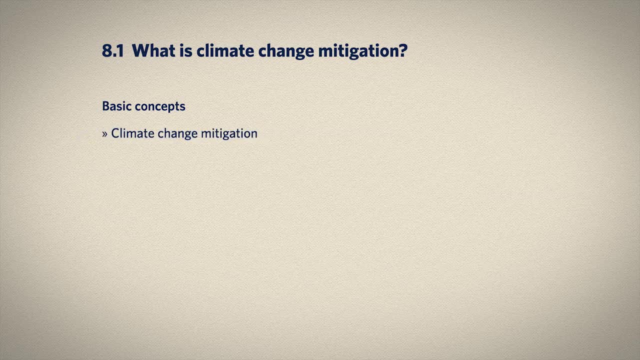 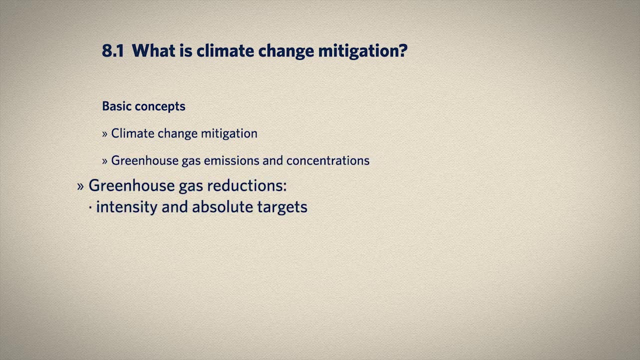 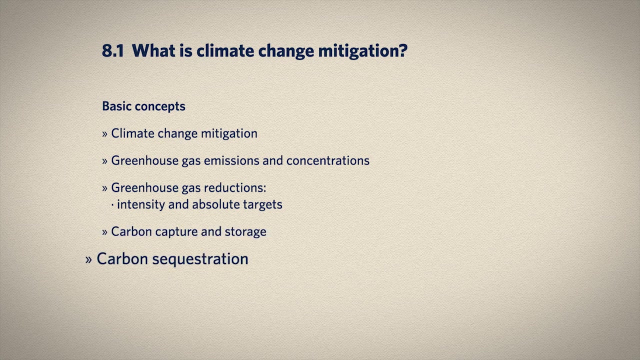 During this lecture, we'll learn the widely held definitions of, of course, climate change mitigation, greenhouse gas emissions and concentrations- which is a refresher from previous lectures- greenhouse gas reductions, including both intensity-based and absolute reduction targets, carbon capture and storage, carbon sequestration and also geoengineering. 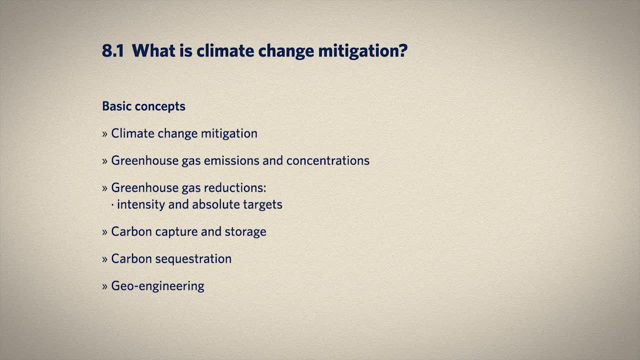 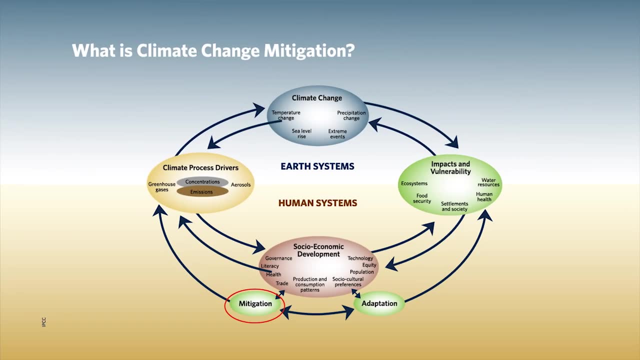 As the first half of this class really has shown, human systems and earth systems are inextricably linked. The ways we choose to develop our cities, grow our food and live our lives has a direct impact on both the quantity of emissions we put into the atmosphere. 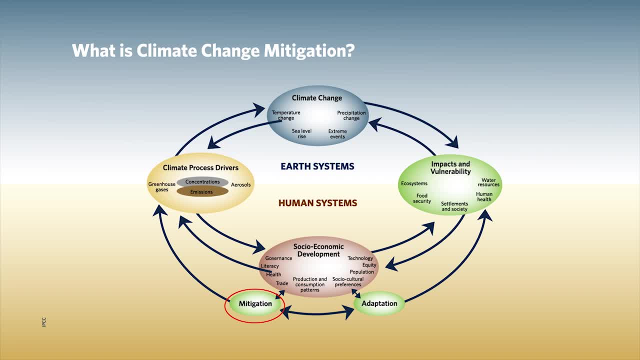 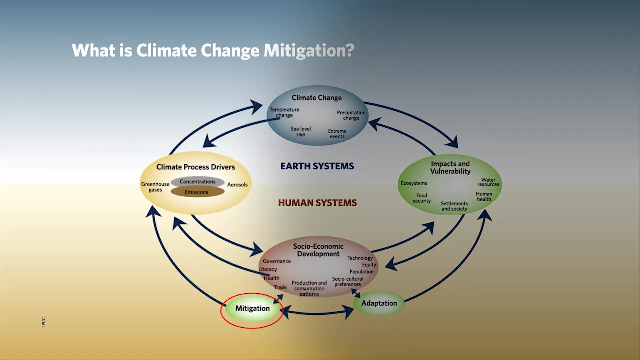 as well as, of course, the level of climate change that we ultimately experience. Similarly, the places we choose for our settlements, for our cities, and the way we build those settlements directly influences our degree of vulnerability to the impacts of climate change. In this module, we're focused on the interactions that occur on the left side of the diagram. 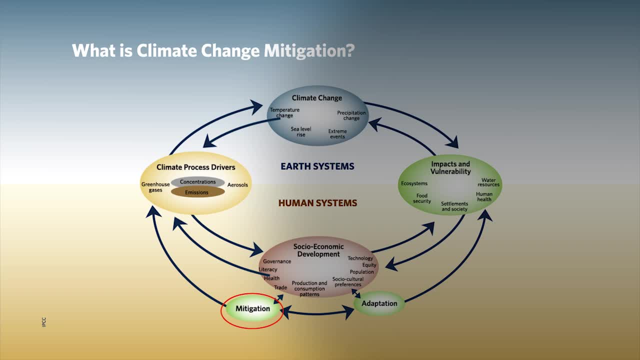 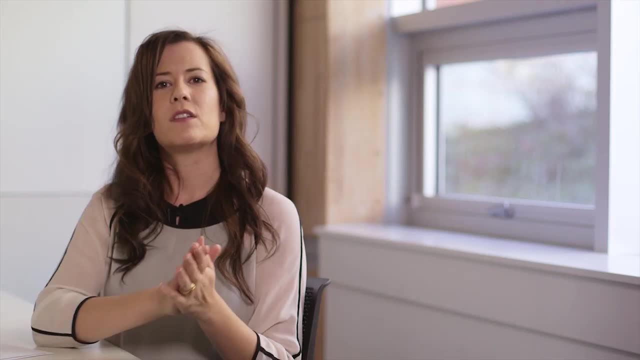 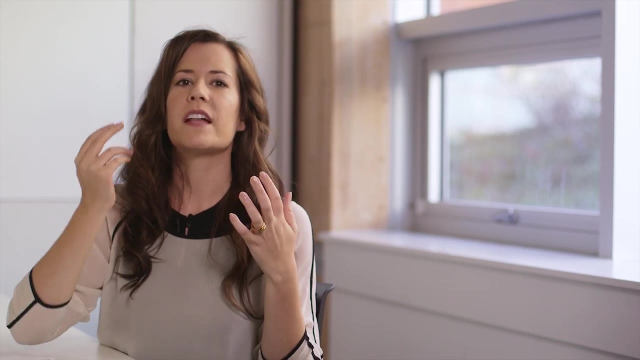 that you see here, with a particular focus on mitigation, and then next week, in module 9, we'll focus on adaptation- the right side of this schematic Climate change. mitigation is another term for dealing with the causes, rather than the consequences, of the climate change problem. In other words, the goal is to prevent climate. 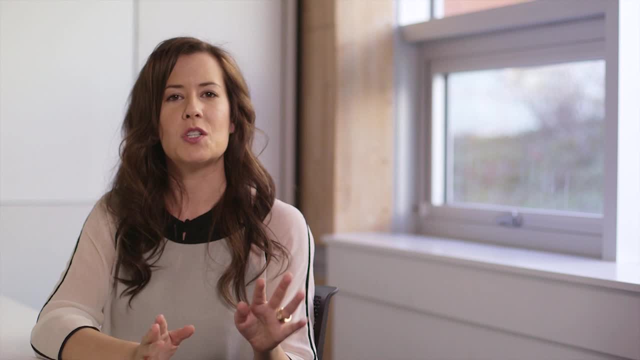 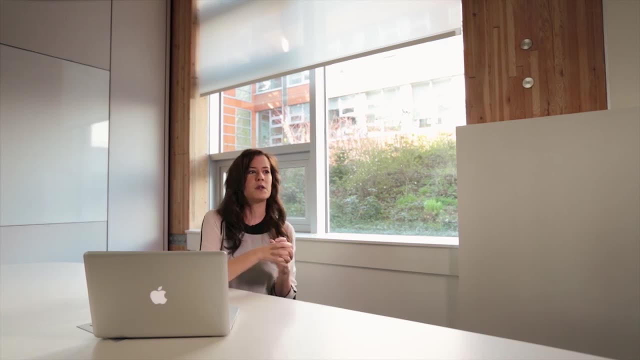 change before it starts, rather than dealing with the impacts of climate change once they've begun. Climate change mitigation has been the most important policy response to climate change since the evidence for human interference with the planet's climatic balance really began to emerge. The reason for this is part. 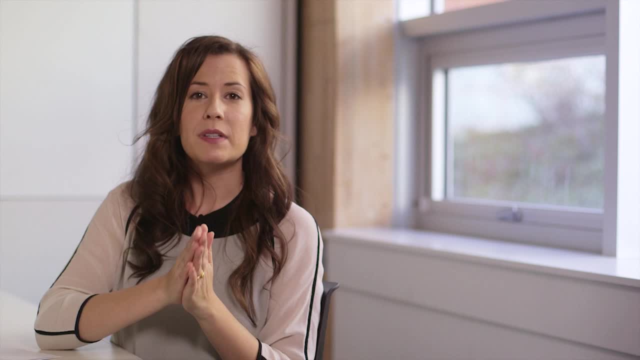 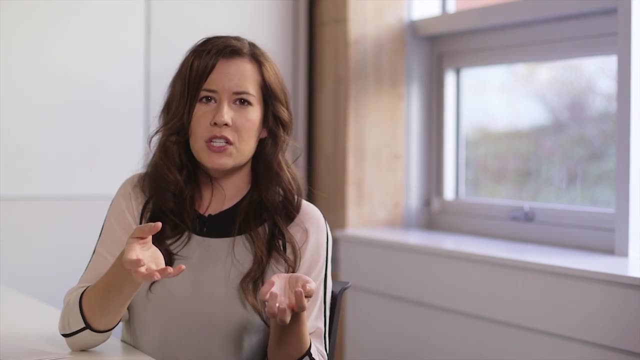 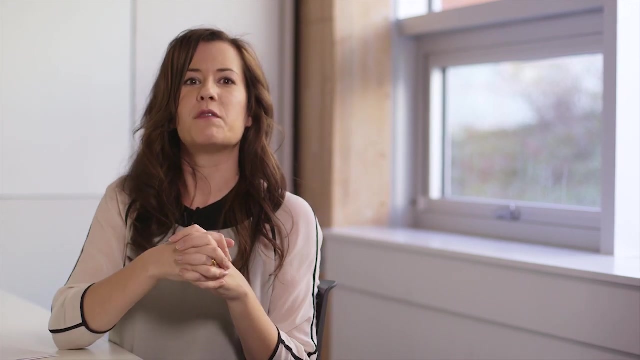 politics and part optimism. Until recently, it's been politically unpalatable to suggest that we'll be unable to sufficiently address the climate change challenge. As a result, adaptation or responding to the impacts of climate change has been viewed by some as an admission that we've failed or will fail to solve the problem of human contribution. 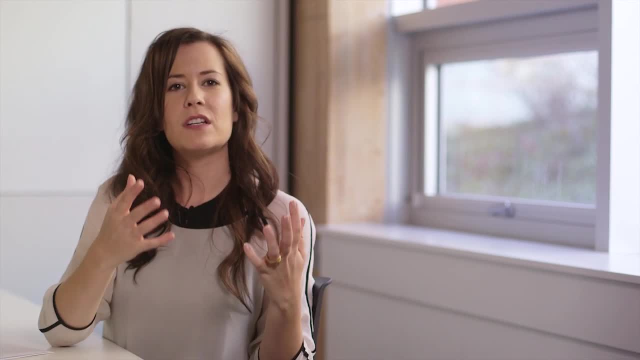 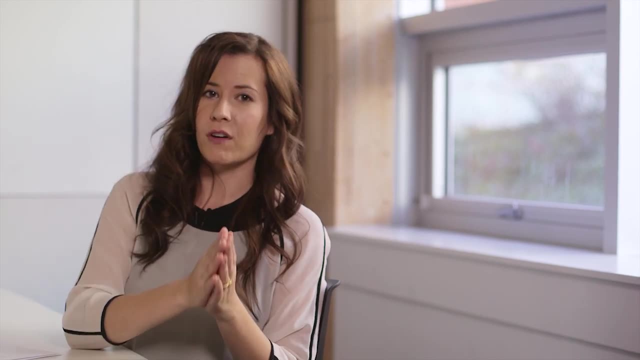 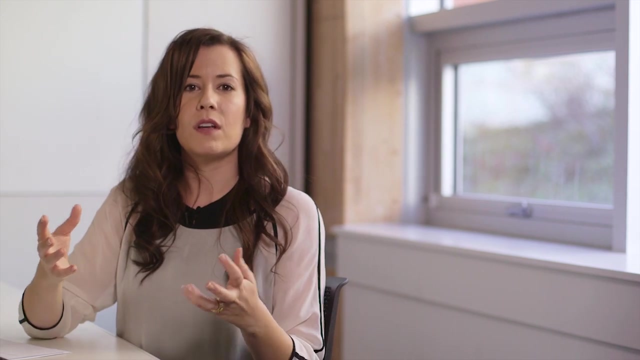 to climate change. The very simple definition of mitigation, based on what we know about the emission of greenhouse gases into the atmosphere, is that mitigation is either reducing our emission of greenhouse gases into the atmosphere or enhancing the ability of the Earth, including oceans and forests, to absorb carbon. 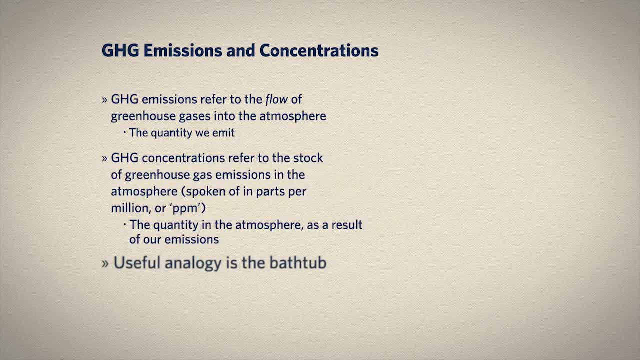 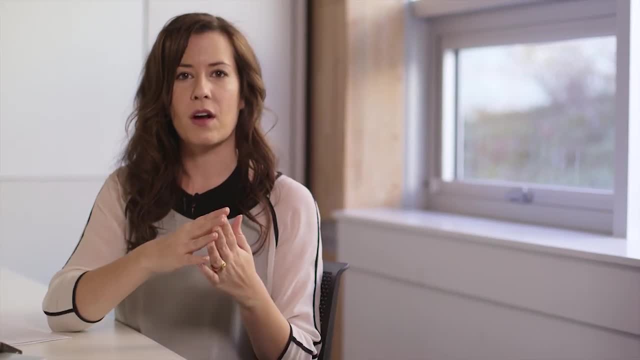 As you've already learned, when we speak about greenhouse gas emissions, we're referring to a flow of greenhouse gases into the atmosphere. The combustion of fossil fuels and the decomposition of organic matter are the primary and most important factors that cause climate change. The greenhouse gas emissions are the primary and most important factors that cause climate. 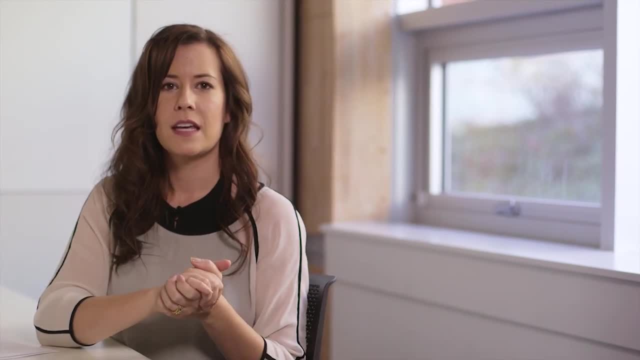 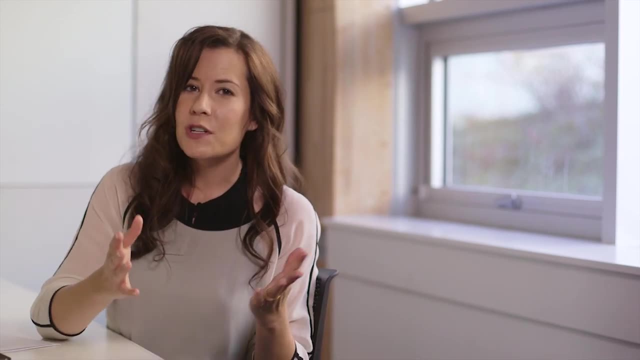 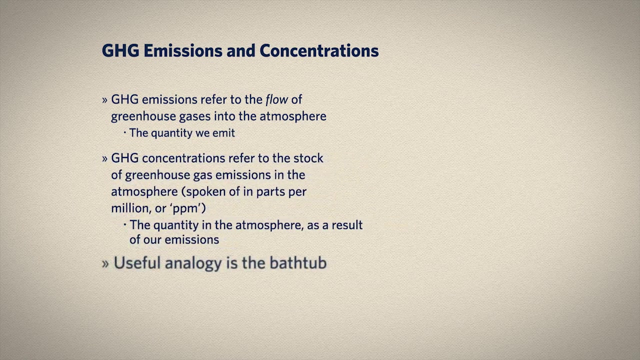 change. This is pushed into the atmosphere by an anthropogenic or human-caused source of greenhouse gases. These result from transportation, industrial processes, residential and commercial heating and cooling, waste treatment and disposal and, of course, agriculture. Greenhouse gas concentrations, in contrast, refer to the quantity of greenhouse gases. 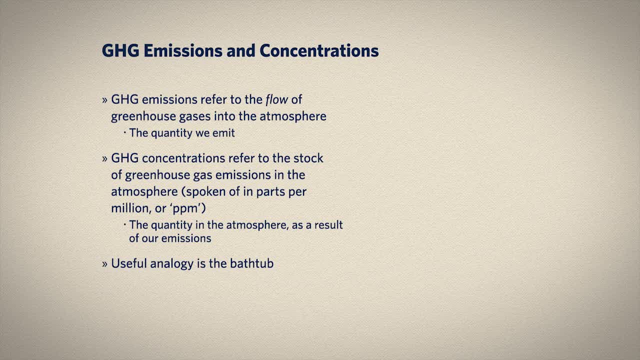 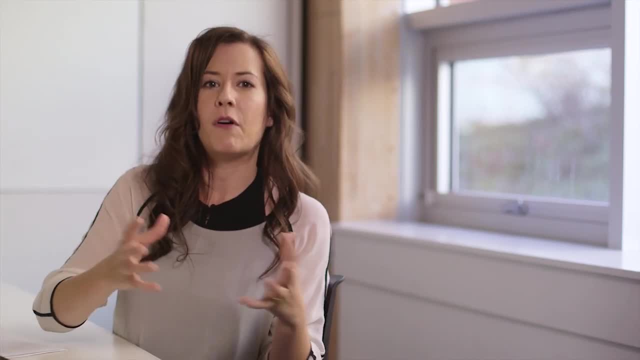 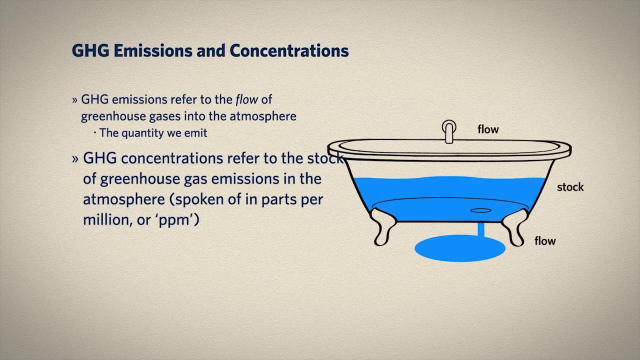 in the atmosphere, a stock, and these are the result of the emissions that have taken place. We often use the metric of parts per million to describe the quantity of greenhouse million units of volume in the atmosphere. how many units are taken up by greenhouse gases? A really useful analogy, I think, for considering these. 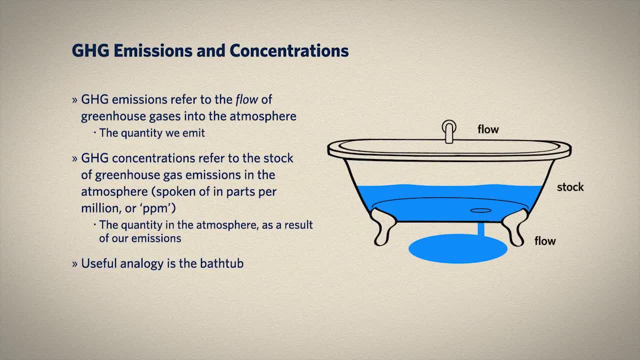 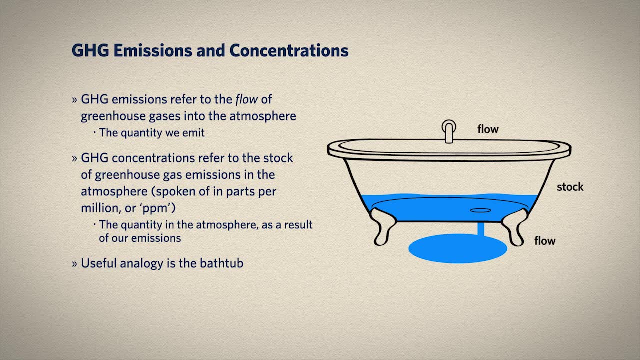 terms is the bathtub, and you've been introduced to this before in previous lectures. We set our greenhouse gas reduction targets based on how full we think the tub should be with greenhouse gases in order to have a stable or a manageable climate. We also set our targets based on the amount of water. 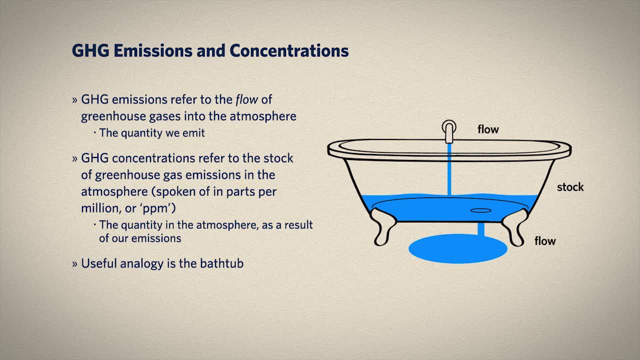 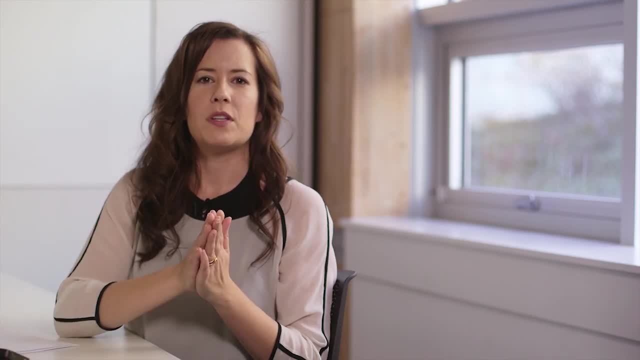 flowing out of the tap. This is how many greenhouse gases we are emitting and the likelihood, of course, that we can reduce these over time. Two key methodologies have been used to set targets for the quantity of greenhouse gas emissions that we are injecting into the atmosphere. The first is called 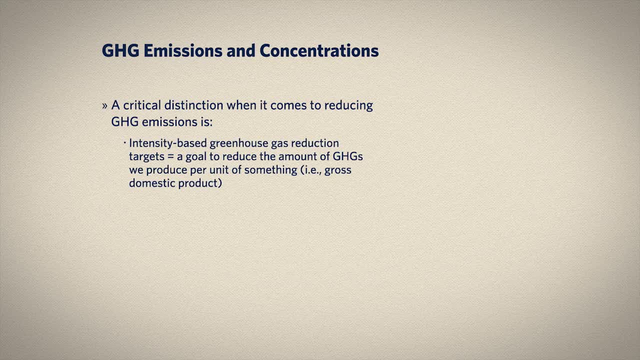 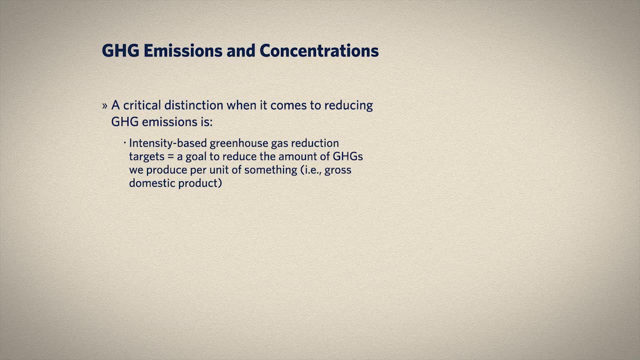 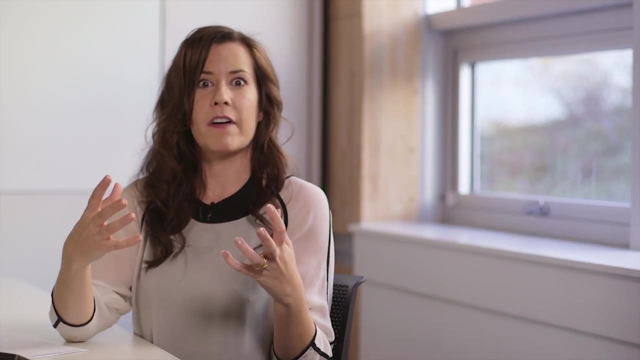 intensity-based targets, and with these we agree to reduce the amount of greenhouse gases we emit. per unit of something, For instance, we might agree to produce fewer greenhouse gases per unit of gross domestic product or per capita. The total amount of greenhouse gases that we emit, though, can go up if I 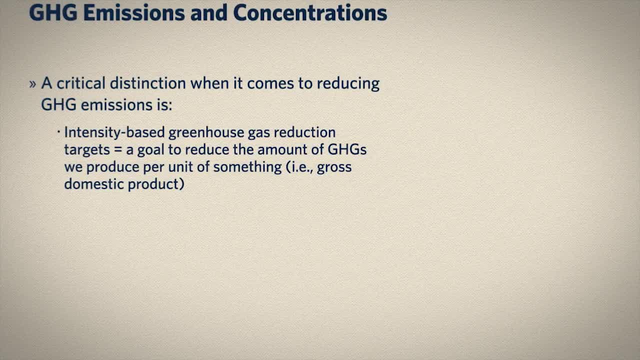 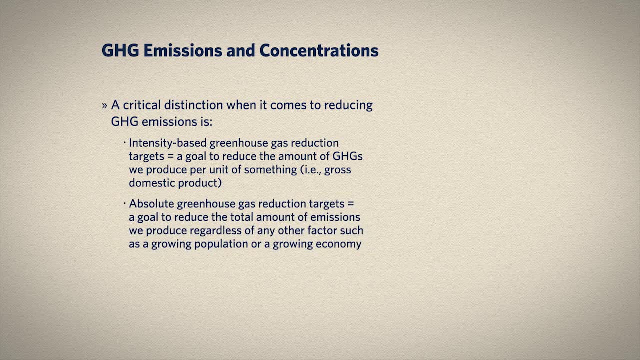 consider the size of our economy or population increases. The second type of greenhouse gas reduction targets is absolute targets. This commits us to reducing the total amount of greenhouse gases either that we are emitting or that are in the atmosphere. An example would be the Canadian target agreed to. 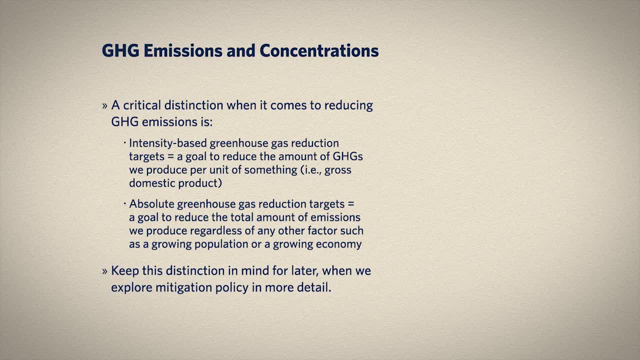 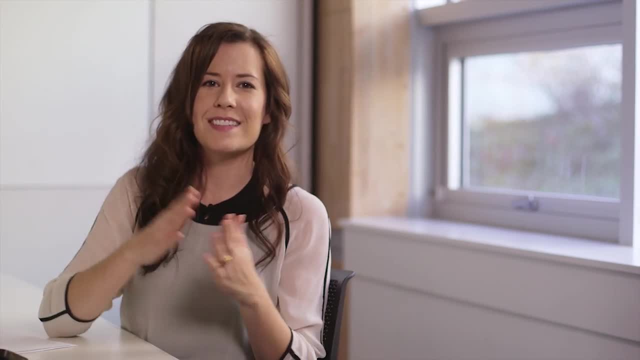 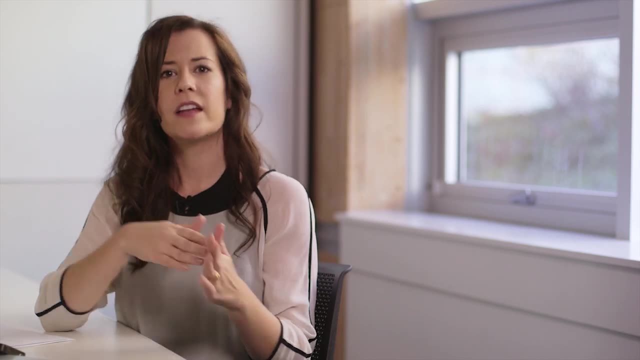 in the Kyoto Protocol and we'll discuss that in a bit greater detail in a later lesson. With the Kyoto Protocol target for Canada, Canadians agreed to commit to reduce their emissions in tons to six percent below 1991 levels between the period of 2008 and 2012.. Another example is the suggestion: 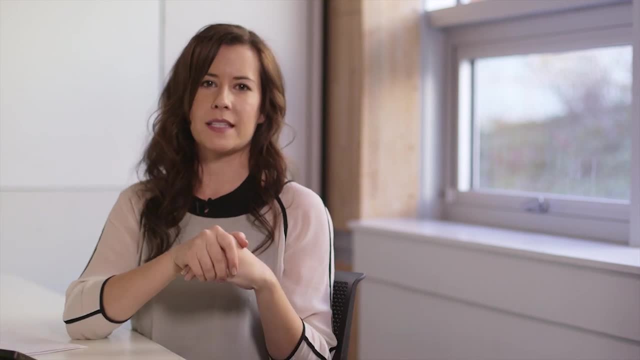 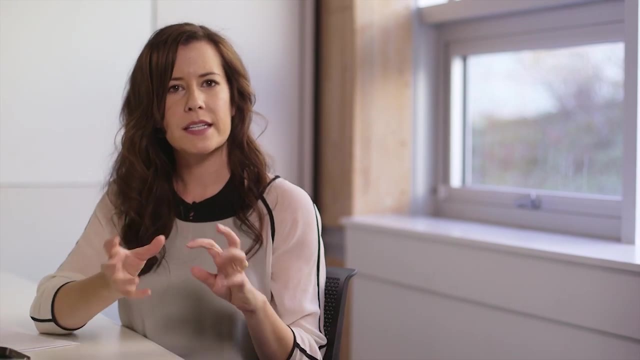 that we should keep the concentration or the stock of greenhouse gases in the atmosphere to 350 or 450 parts per million. This distinction between intensity-based and absolute greenhouse gas reduction targets will be important later in the course when we discuss the various policy tools that are at our 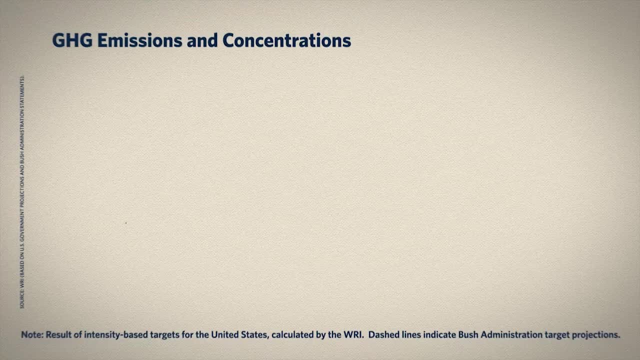 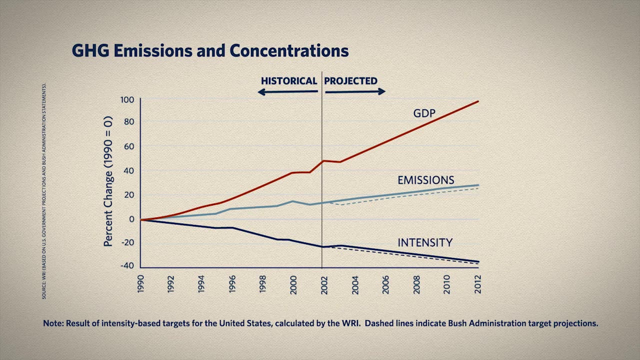 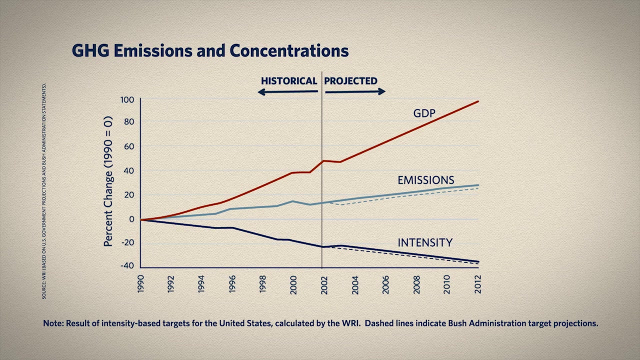 disposal to mitigate climate change. The graph that you see here illustrates the controversy behind intensity-based emissions reduction targets. The horizontal axis represents time going out into the future, and along the vertical axis we see the percentage change in greenhouse gas emissions. As you can see, despite declining greenhouse gas intensity or a 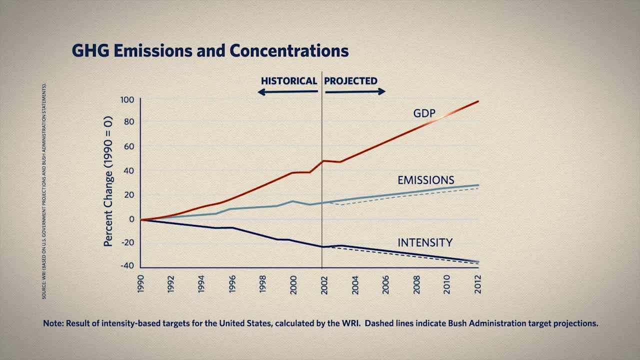 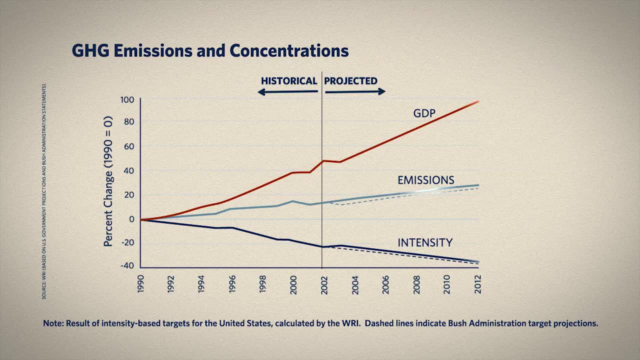 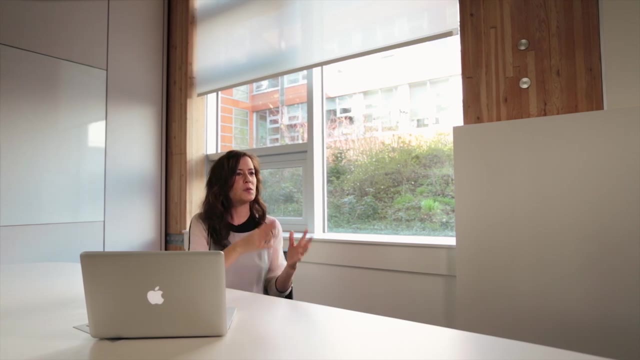 reduction in the amount of greenhouse gases produced per unit GDP. GDP is still rising so quickly at such a rate as to cause overall absolute emissions to still increase. As a result, these intensity-based targets wouldn't really be expected to contribute as much as we'd like to the 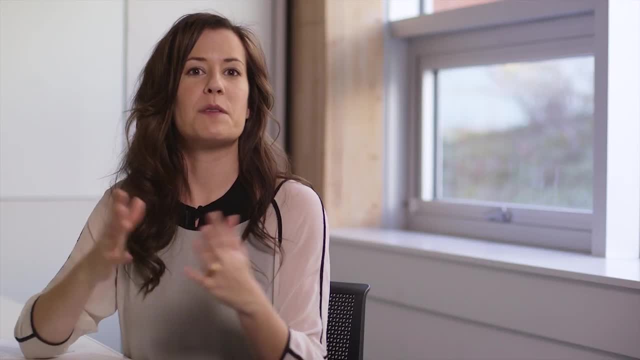 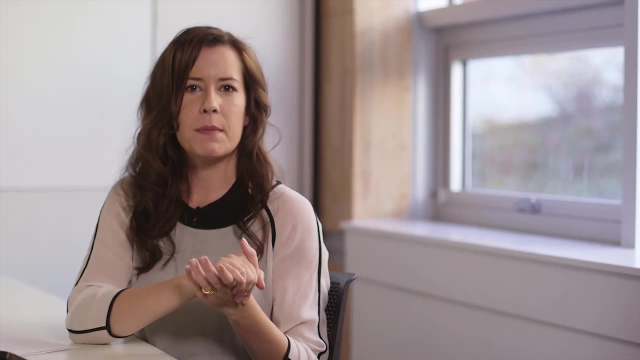 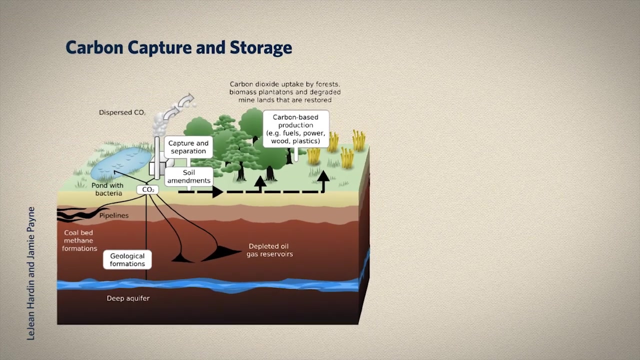 prevention of climate change impacts. Before we move on, take a moment to answer this quiz question. In addition to reducing the quantity of greenhouse gases that we emit, we can also enhance the quantity of carbon taken up by the planet in order to mitigate climate change. This is the idea behind carbon capture and storage. We 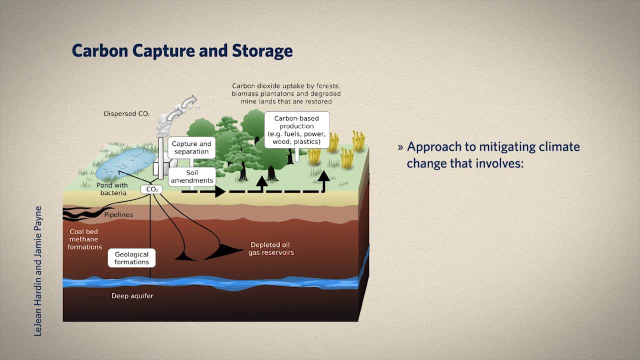 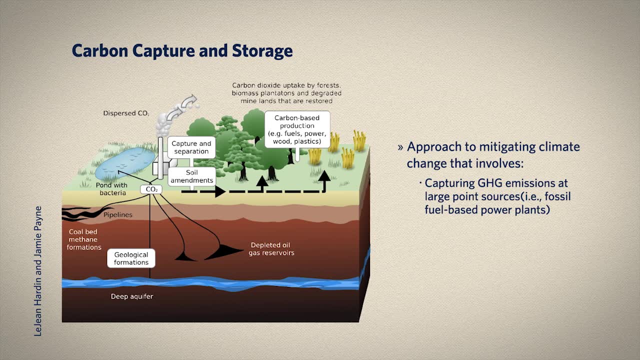 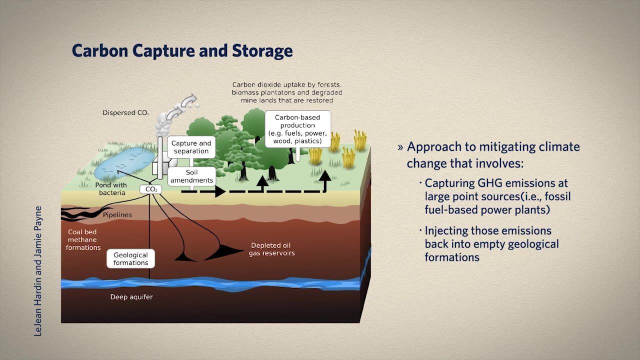 still burn natural gas to heat our homes or use electricity from a coal-fired power plant. But instead of venting that carbon dioxide that results from the combustion process into the atmosphere, we capture it and we store it. Proposals and ongoing projects have been made to inject this captured carbon dioxide into 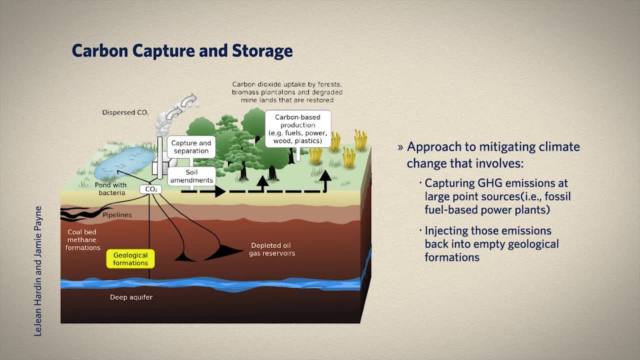 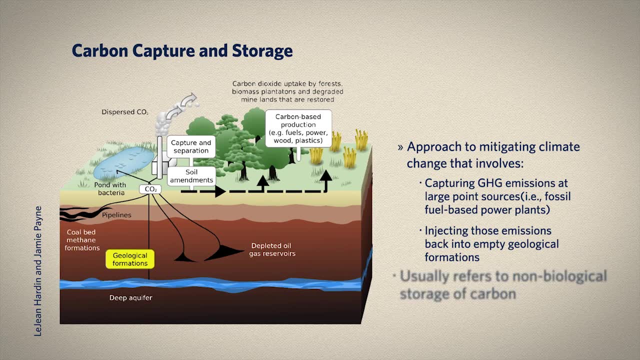 geological formations that contain empty spaces after oil or natural gas has been extracted from them, The geological formation would be filled with carbon dioxide and then capped. As a result, these greenhouse gases would never make it into the atmosphere and therefore would never influence the climate. 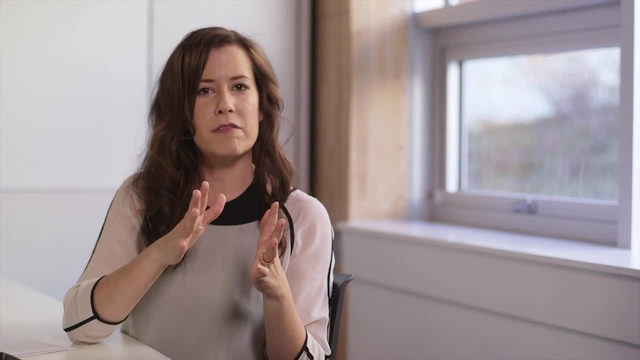 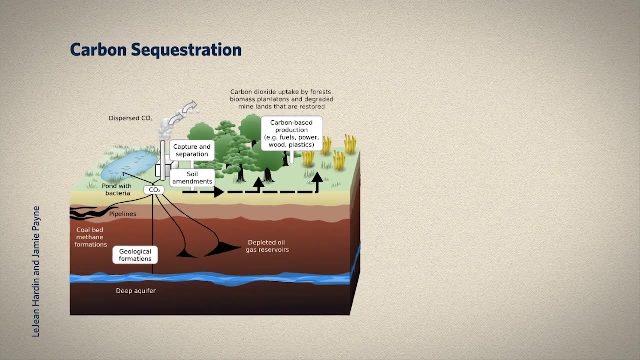 As you can imagine, the idea of carbon capture and storage has created some pretty fierce debate, and we'll discuss the nature of this debate in a little bit greater detail later in the module. The next category of climate change mitigation strategies that we'll introduce is carbon. 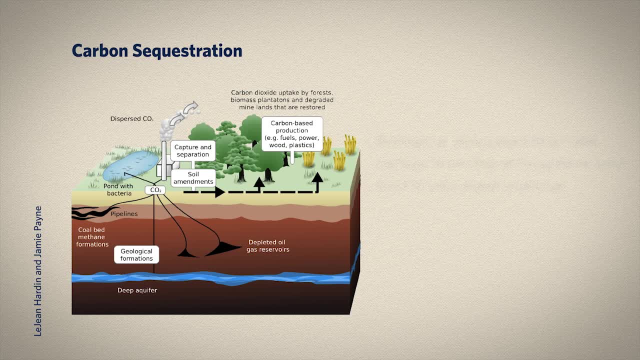 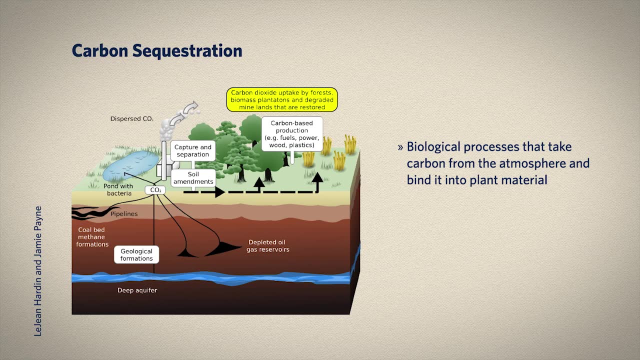 sequestration, So like carbon capture and storage, carbon sequestration involves taking carbon out of the atmosphere after it's been produced through fossil fuel combustion or organic matter decomposition. In contrast, carbon sequestration involves the capacity of photosynthesizing.